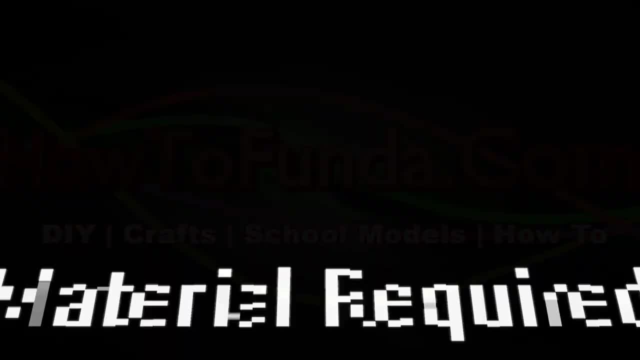 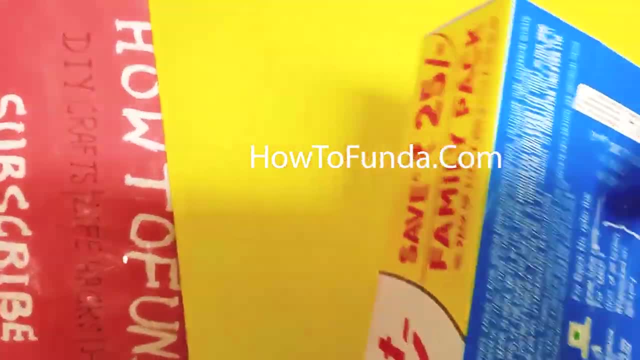 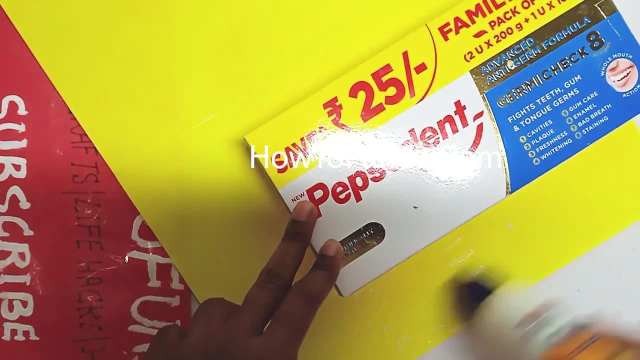 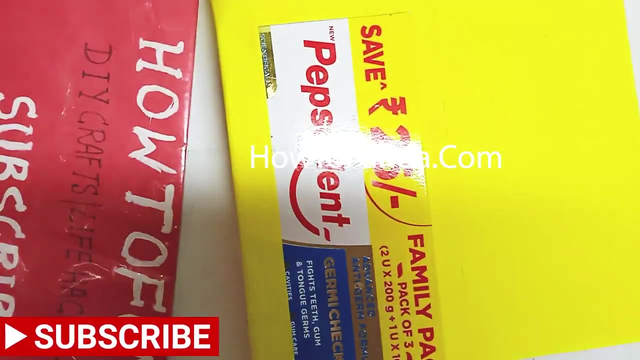 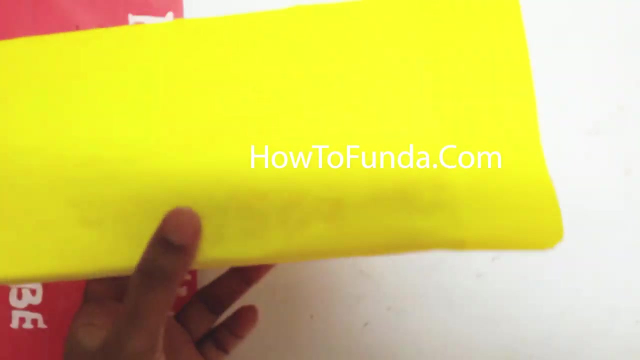 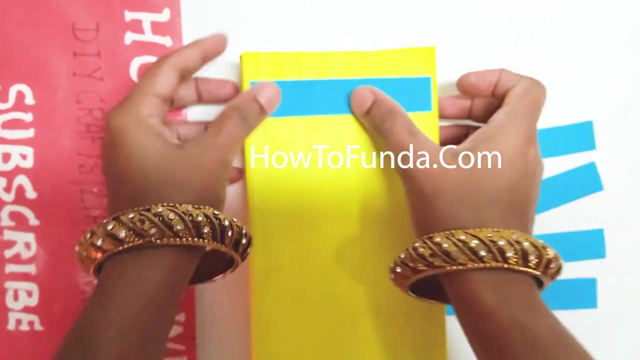 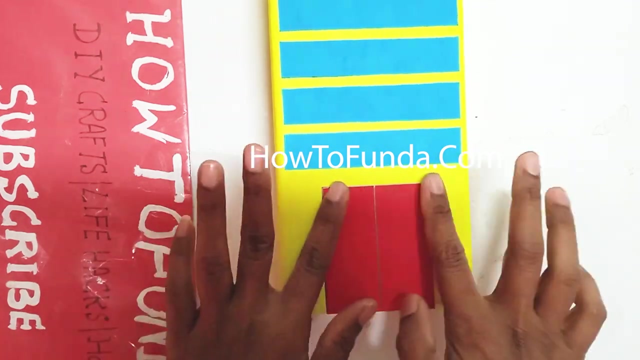 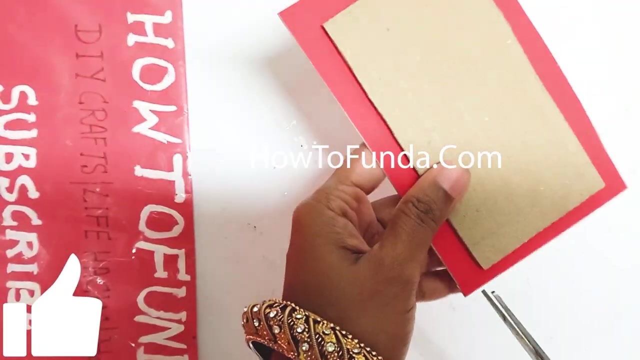 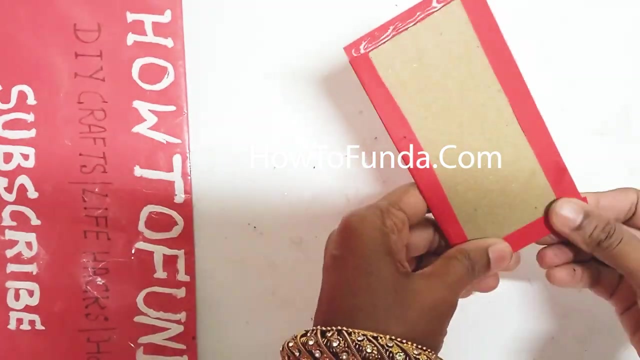 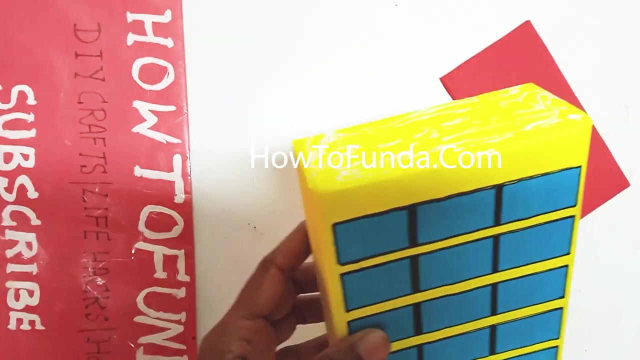 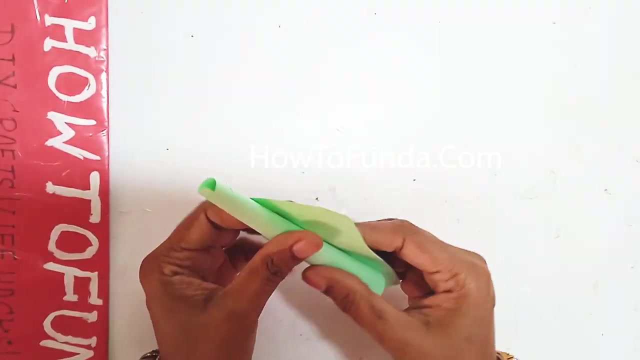 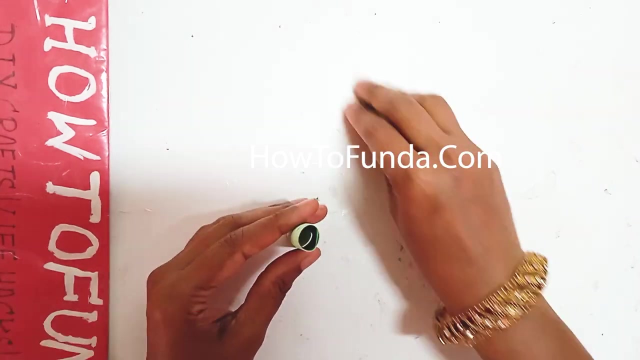 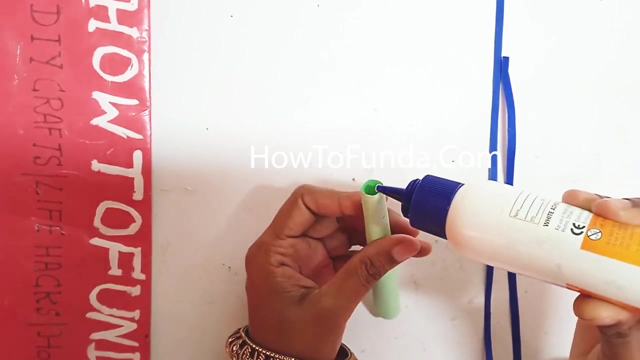 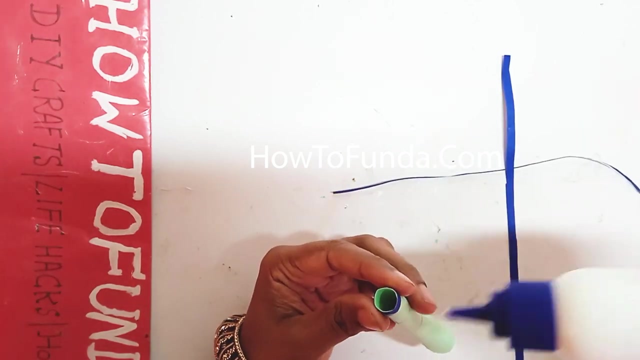 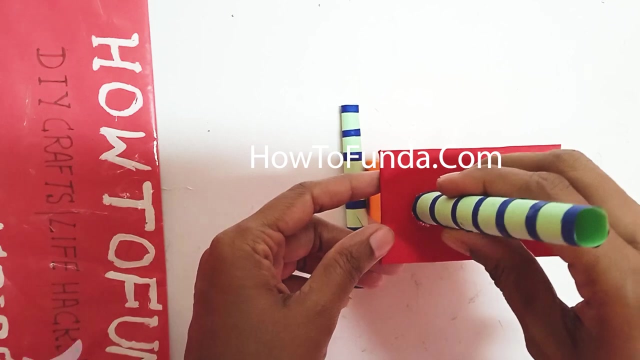 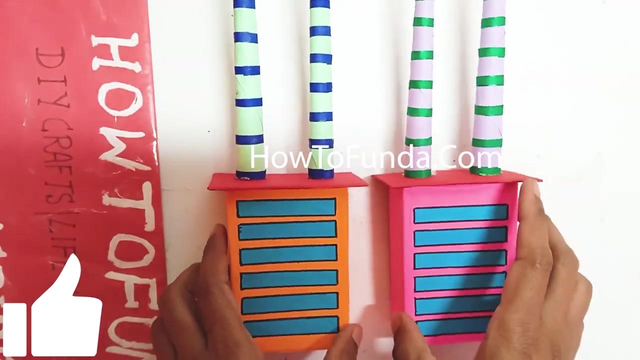 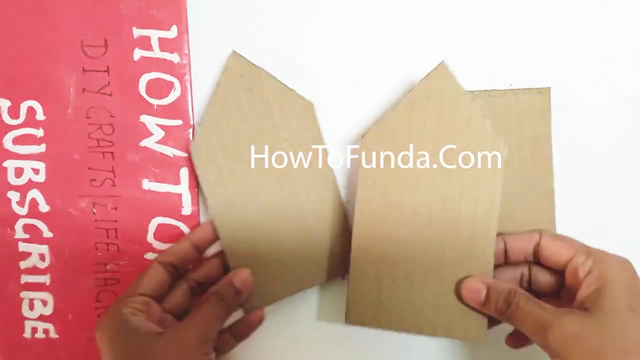 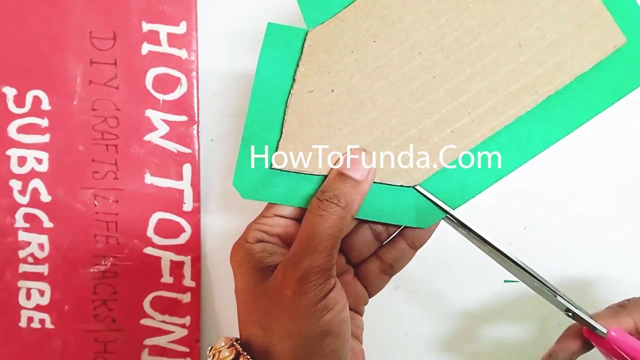 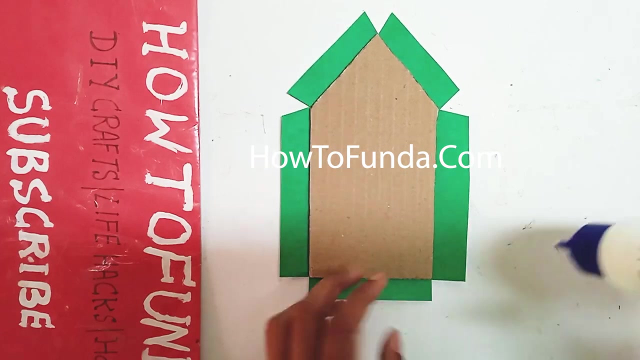 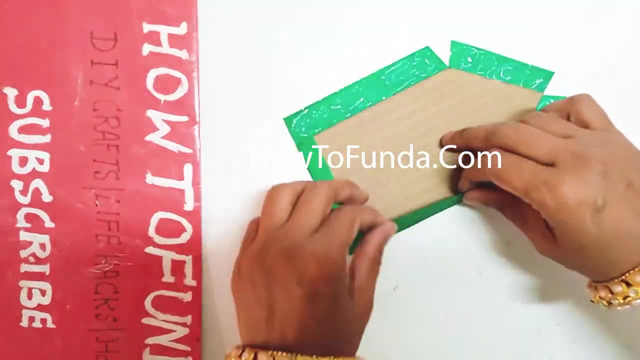 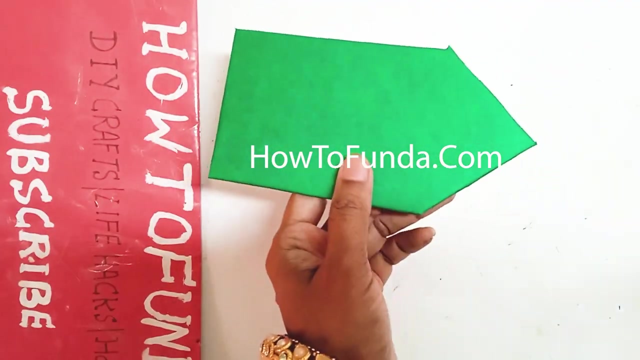 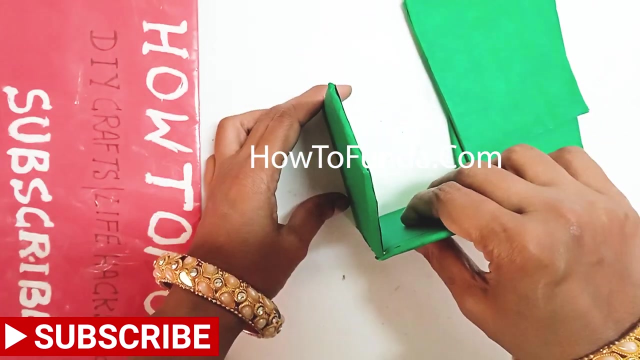 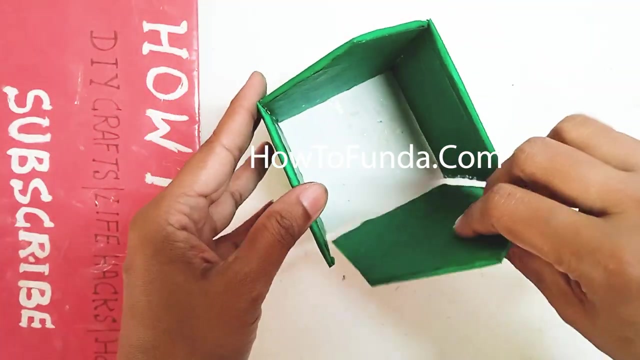 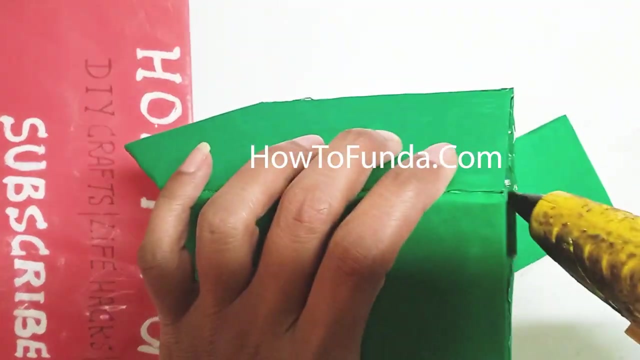 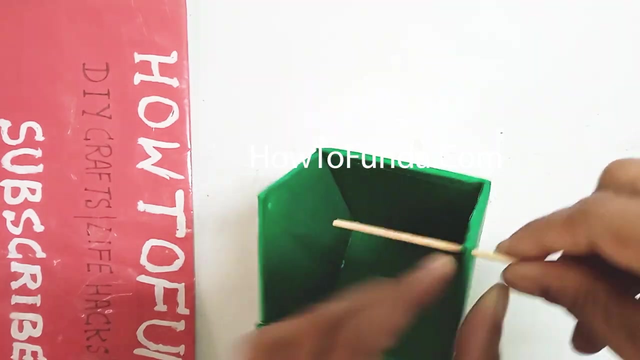 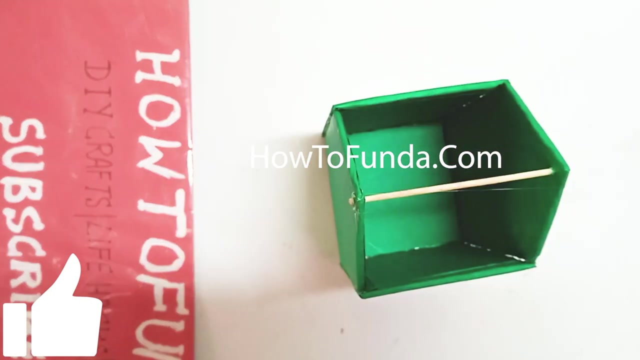 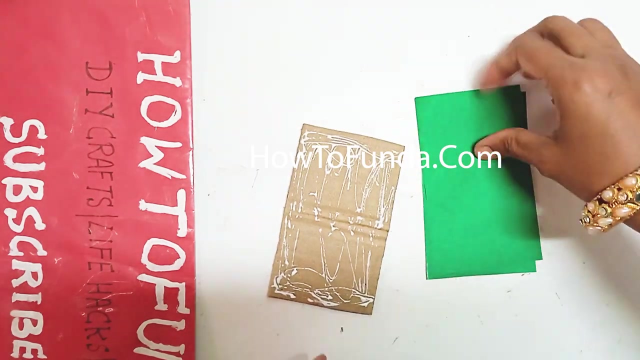 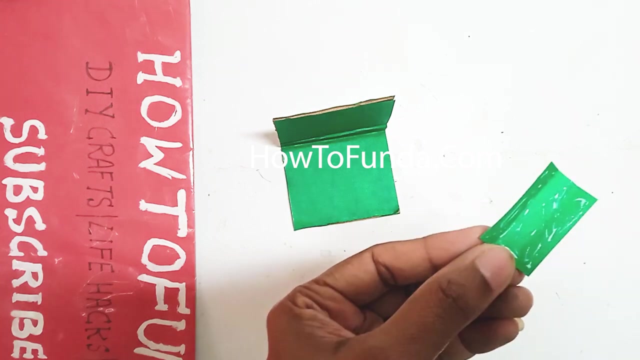 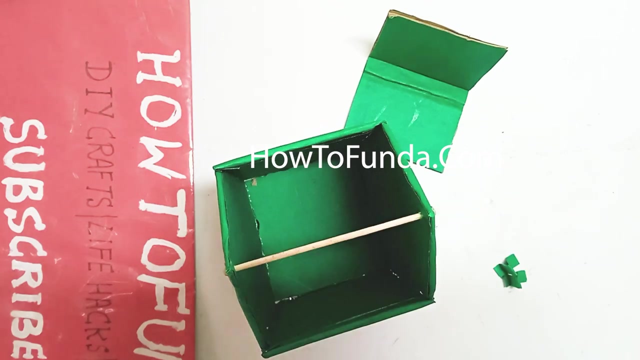 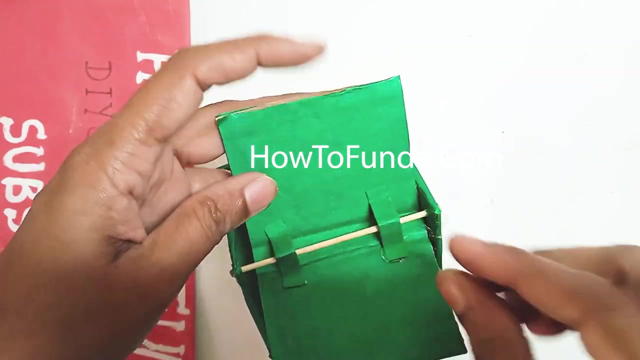 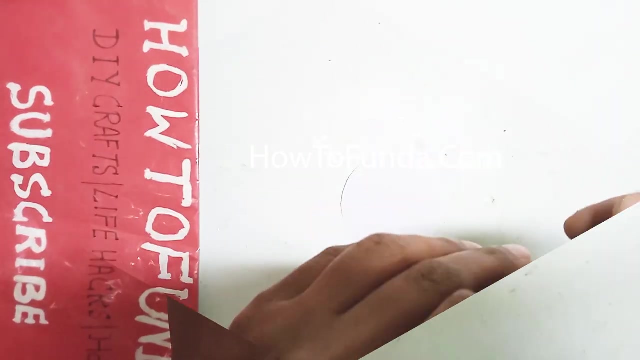 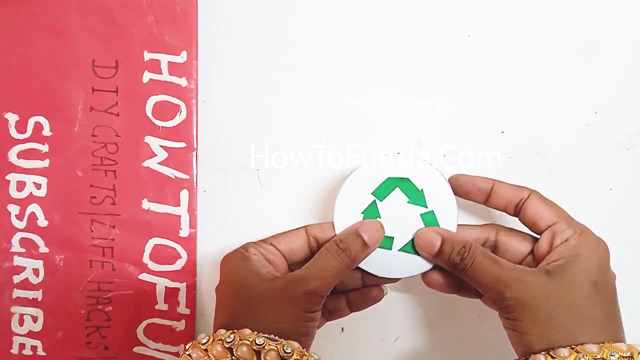 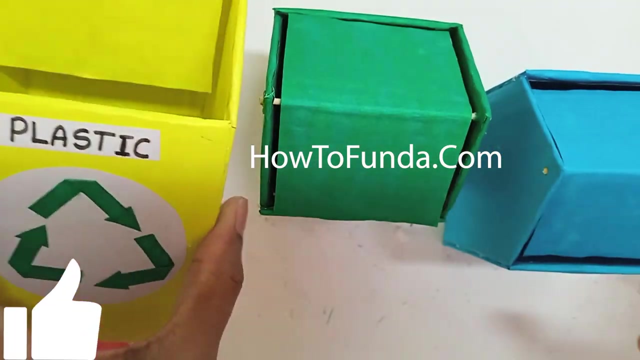 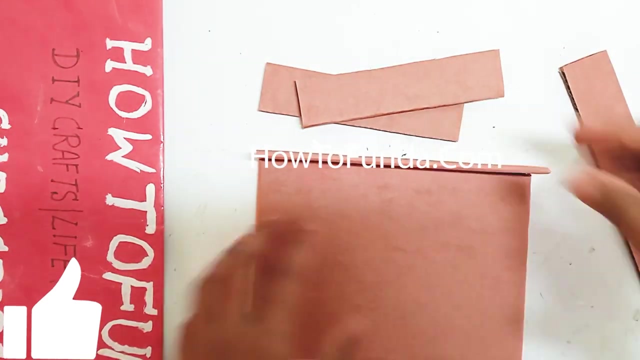 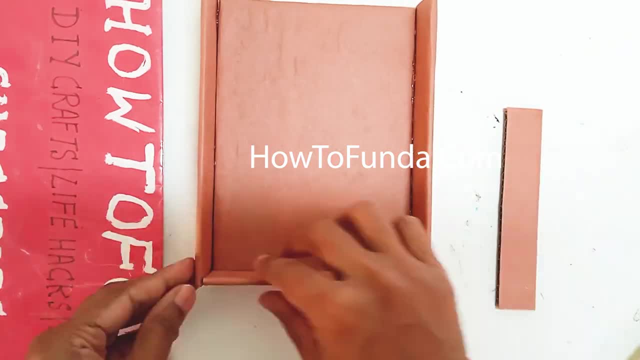 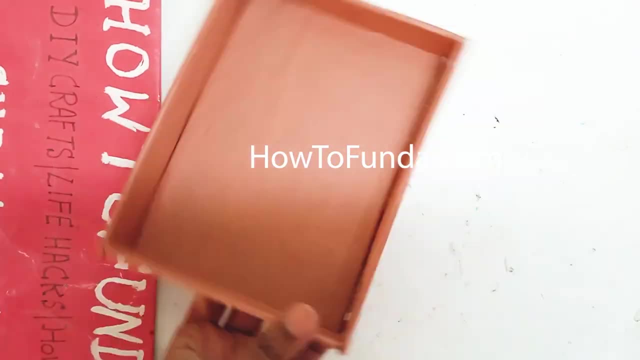 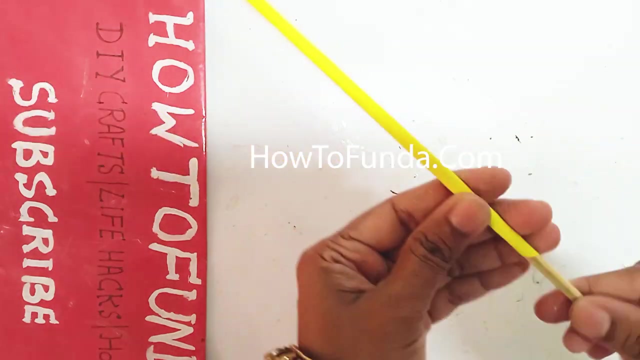 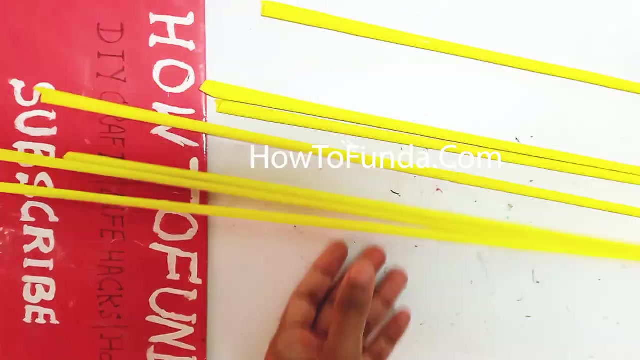 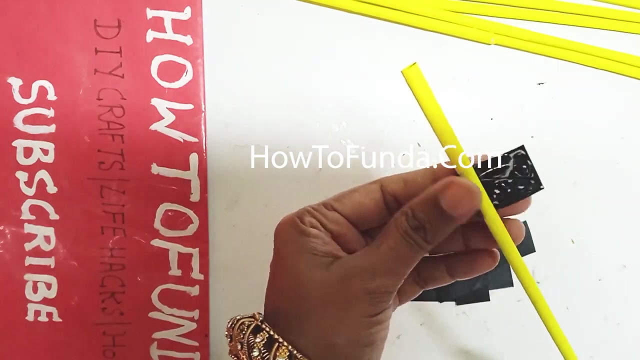 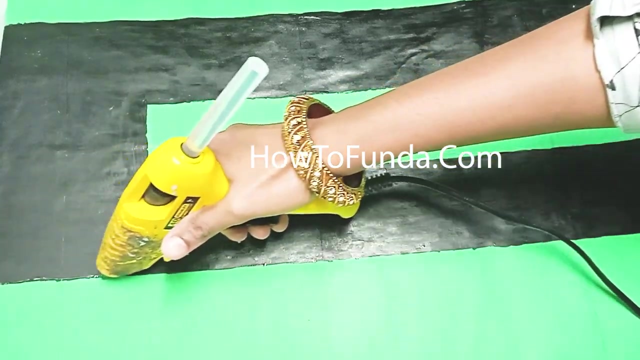 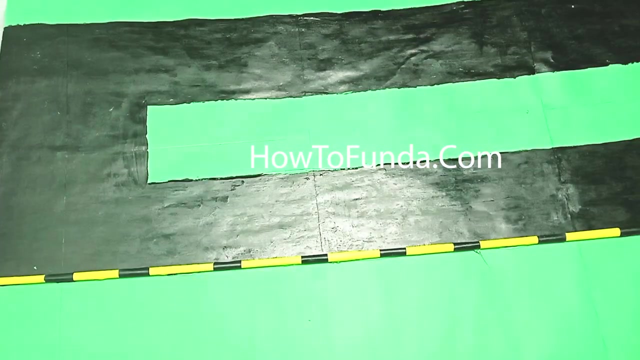 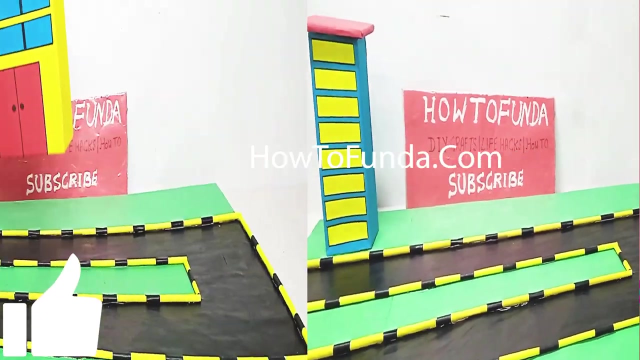 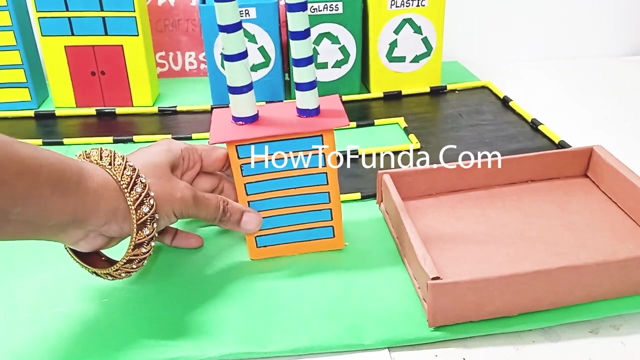 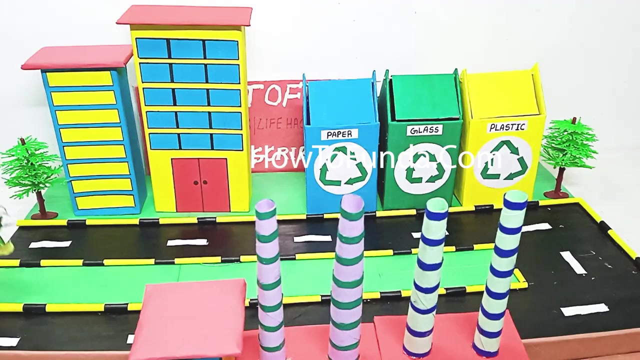 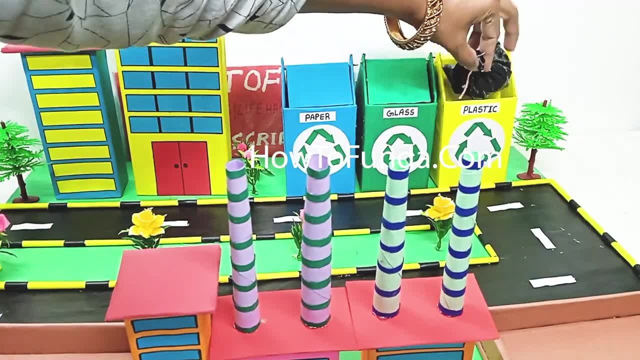 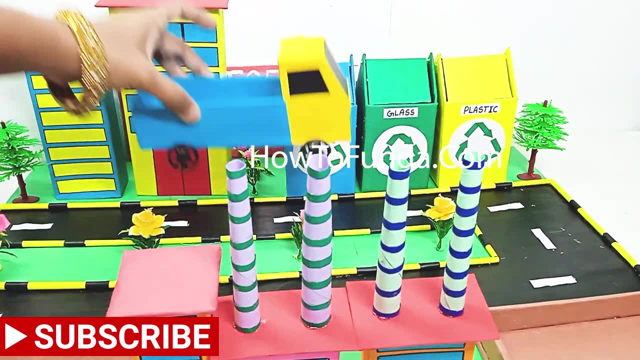 Of everything you know that you could get. Don't let them guide your life towards regret. A fight for what I love with every breath. My past is filled with things I won't forget. I used them all to push me to my best, So I won't forget you. 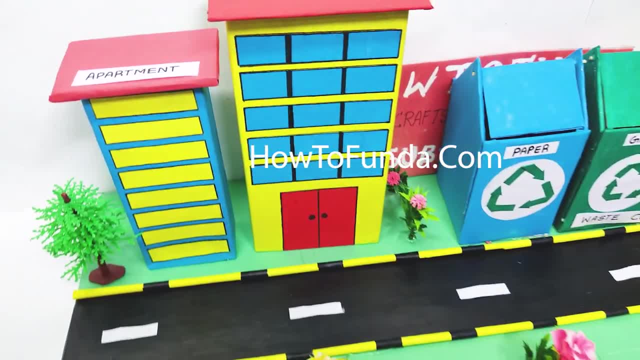 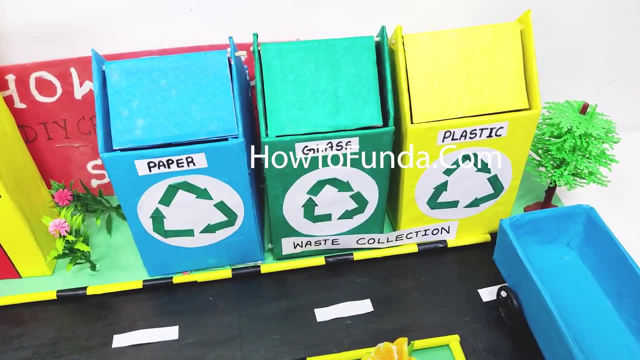 So I won't forget you. We'll treat the worst of times just like a test. If only I could go back in time. I tell myself that everything will end up alright. Just push yourself, test yourself, figure out what you like And find your limits. don't be rigid. always work towards a prime. 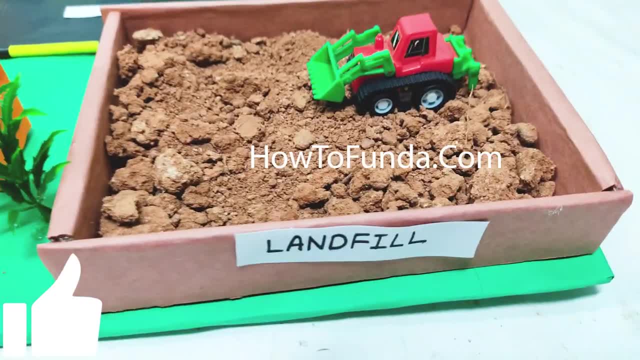 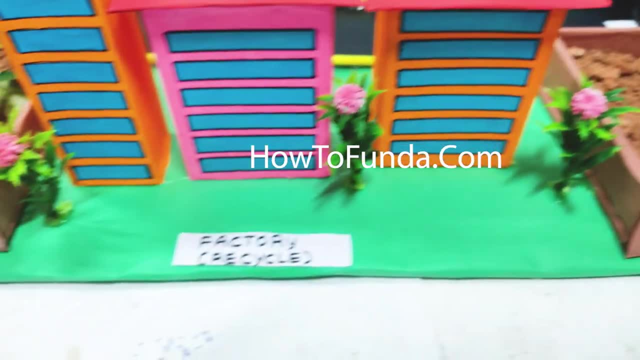 Surround yourself with open minds. people can't change your life. A few friends with intent can help you feel alive. Find a passion, take some action and, with a little time, Just be patient. make a statement. try to enjoy your life. They'll try to kick you while you're down. 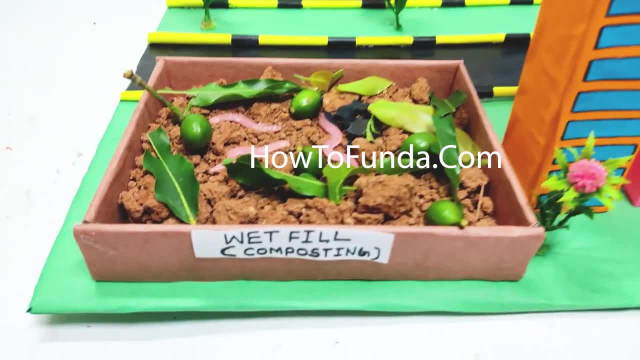 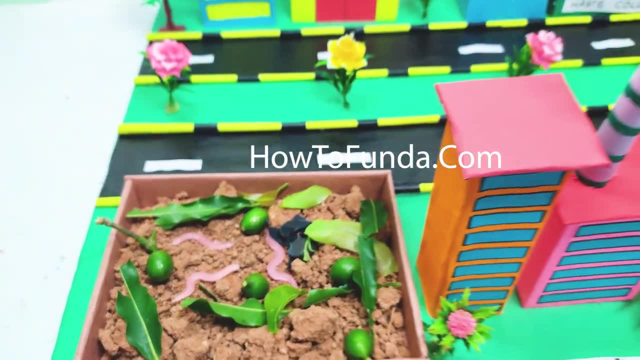 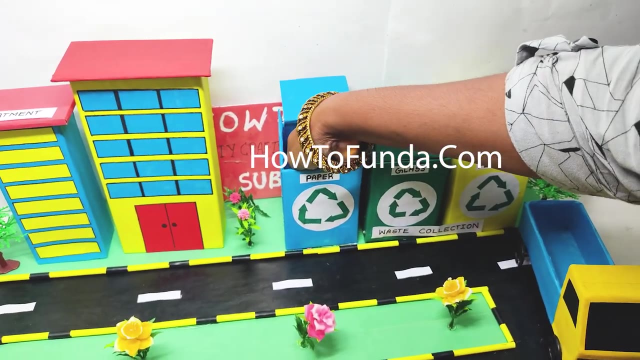 They wanna rise up while you drown. They wanna fill your head with doubt. They're silently scared that you'll figure it out. I'll make you look like I'm losing, Won't bother hiding my bruises. And when they finally think you're wounded, Then it's your chance to be ruthless.